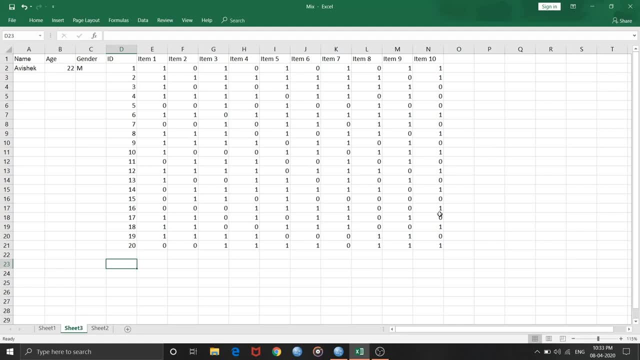 Now there is this popular section. The suggestion by Kelly in 1939 says that best strategy is to select upper 27% and the lower 27% of the respondents And then within these two extreme groups of scorers we will see how much the item is discriminating or not. 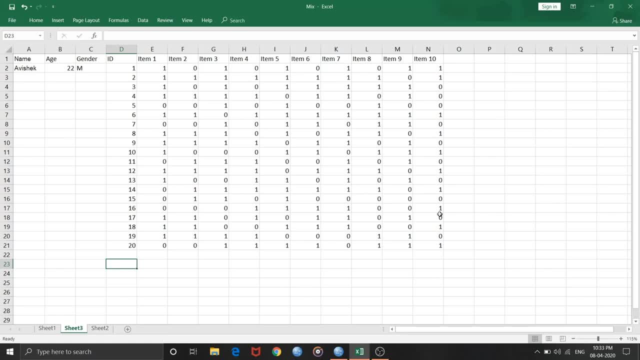 And for that you need to have total for the items, like total score for the items. Now in this fictitious data you can see that I have 10 items and there are 20 respondents in total, And for that you need to have total for the items, like total score for the items. 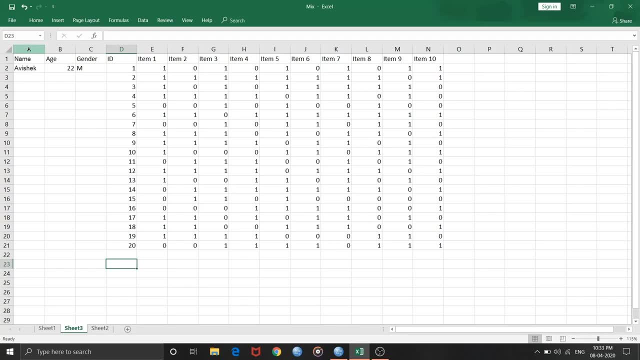 Because I am placing columns for data. We'll see them in theредfts file. So there you can see. in the first column I have the name of the respondents, casual gender id and actual responses for the items from this until this last cell, the range. 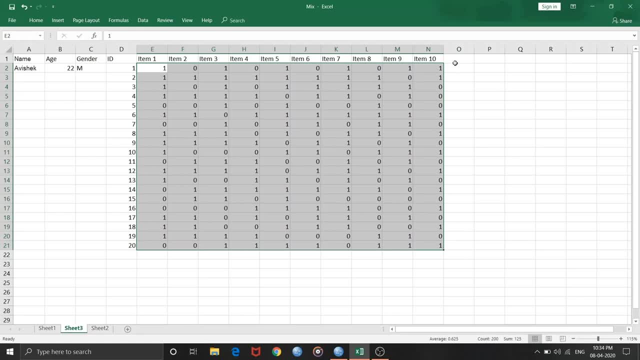 Now firstabhishek is the anonymous respondent in my fictitious data. Now I am interested in finding out total scores for all the respondents in order to arrange them in descending order. descending order: that is required to find out first 27 highest scorers or and lowest score. 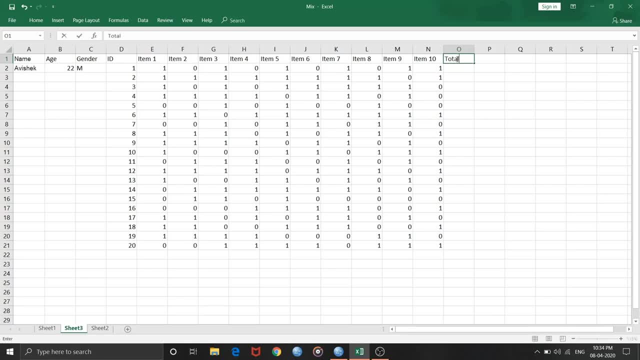 27 percent of scorers, so that i need to do so. for this, i'll use formula of equal to sum summation and double click on that and select these values. give me total for my first respondent and if i drag this down, i'll get it for all the respondents. now i need to arrange this. 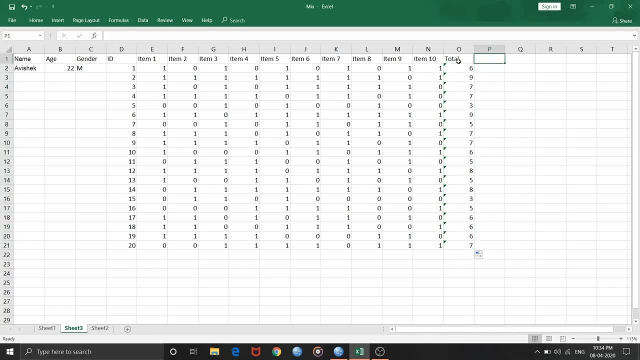 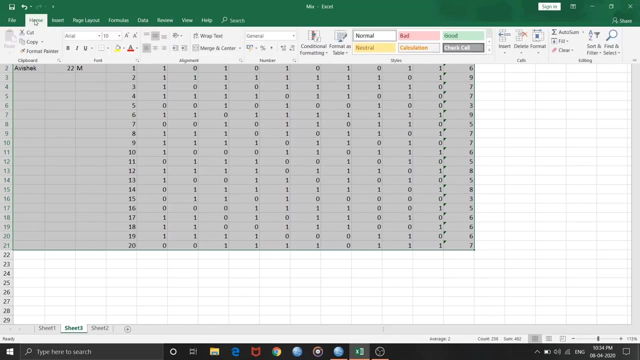 uh, entire data in descending order with respect to total scores of the respondent. so in order to do that, i'll have to select the entire data. once i select that, i'll go in home. on this top ribbon you can see that i have home as an option and in this i have this sort and 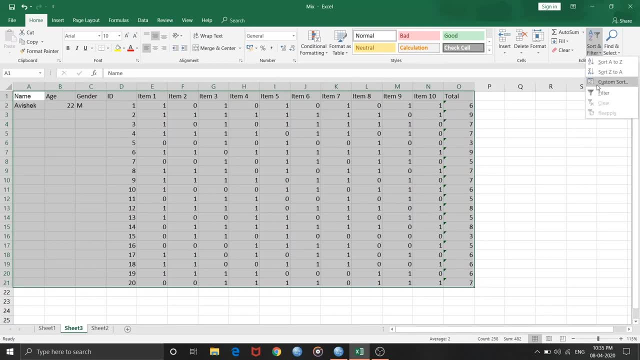 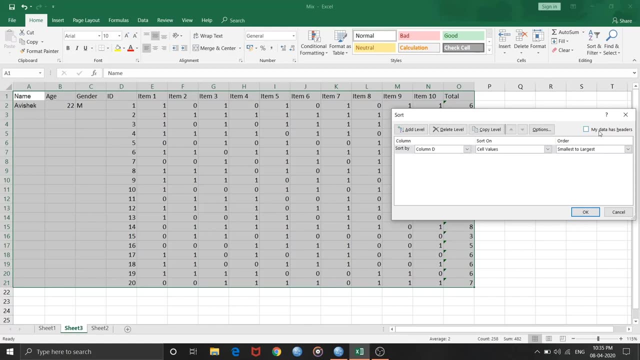 filter option over here. once i click on that, i'll go for custom sort and in this, uh, there is a small my data has headers option. so make sure that, uh, you click on that or check on that, so it will give you sort by options over here. and now you can see that i can sort by all these headers, so i need to. 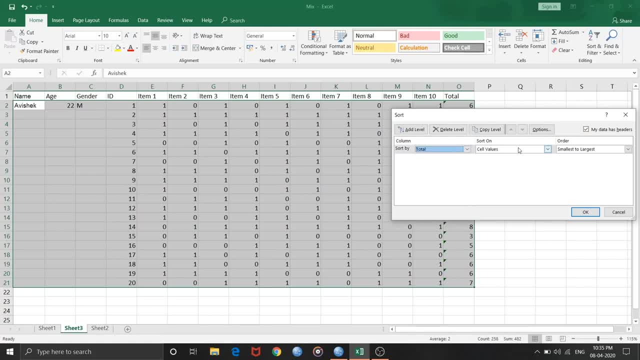 sort my data with help of total scores or with respect to total scores. so and then that will be from largest value to the smallest value in descending order. i'll click on ok. this will sort my data. now you can see that my first respondent is no longer first one respondent, but 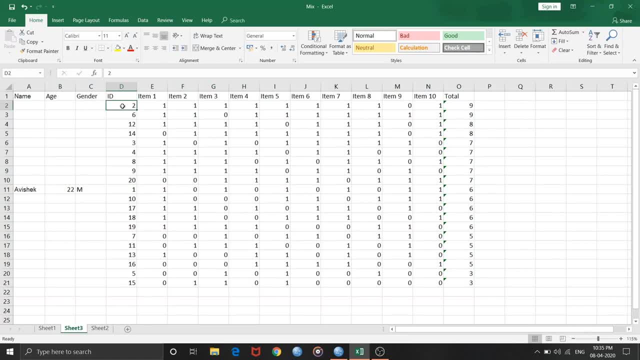 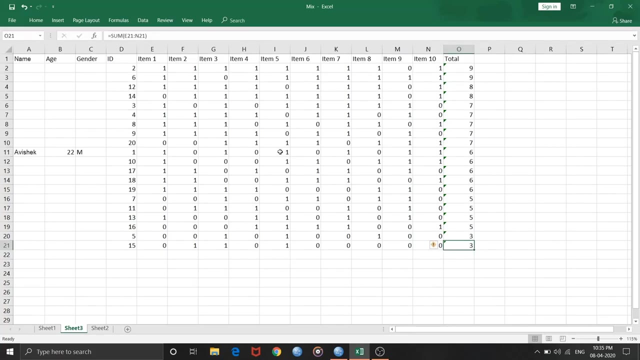 it will be first respondent and the highest scorer is second and sixth respondent respective. like both, both are scoring actually the same value, nine, nine, whereas lowest scorers you can see three is the lowest score on my scale. now i am interested in finding out the um number. 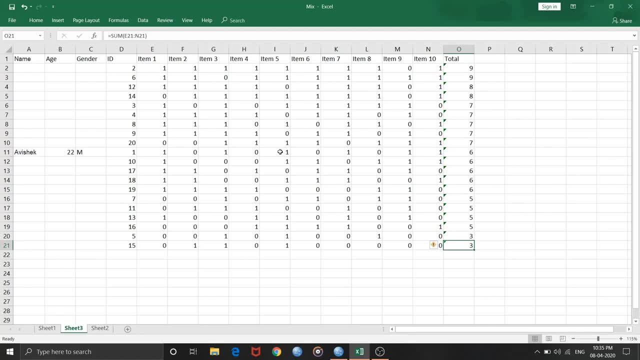 of respondents that will be there in the first 27 percent of respondents. now in my data, as you can see that i have total sample size of 20.. so 27 of 20 are 5.4. now i can either go for 5 or 6. i can't have a decimal in my total, like in number. 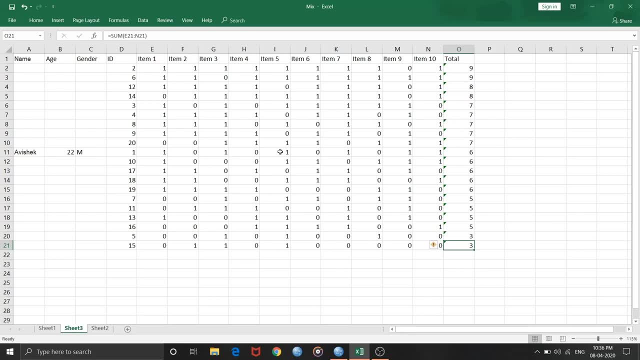 of cases. cases will be a whole number. so in in this particular case, i can either go for 5 or 6. if i go for 5, that will be 25 percent of my total sample. so first 25 percent, in the last 25 percent. 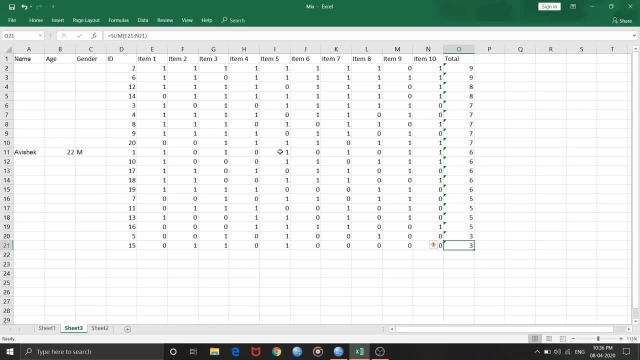 i can see, or if i go for 6, there will be 60. sorry, that will be 30 percent of my data. so 30 first 30 percent respondents and last 30 percent respondents i can compare with. so now this is a close call and 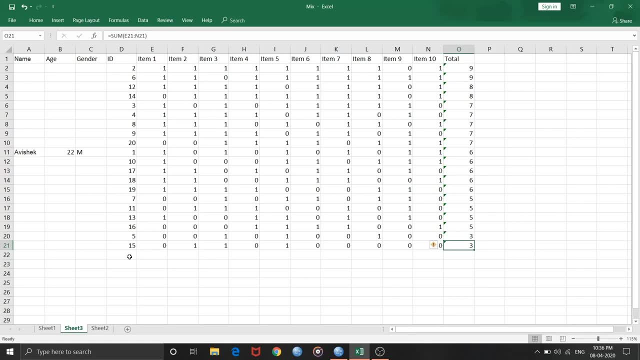 it is all up to you to select that number. so particularly i can, i'll go for 30 for my convenience. so i'll write upper 30. that is first 30 respondents. then i need lower 30, that is least scorers, least 30 percent of scorers, and then i'll be interested in computing di. that is nothing but. 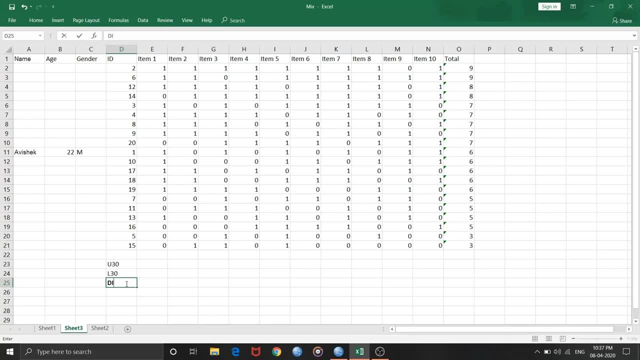 this discrimination index, that is item discrimination basically. so item discrimination: each item will have its own unique value of discrimination may not be unique at times for both, for couple of items can even be same. so, and for all the respondents, if you have that will be called as index. so discrimination index, i will call it as now. i'm interested. 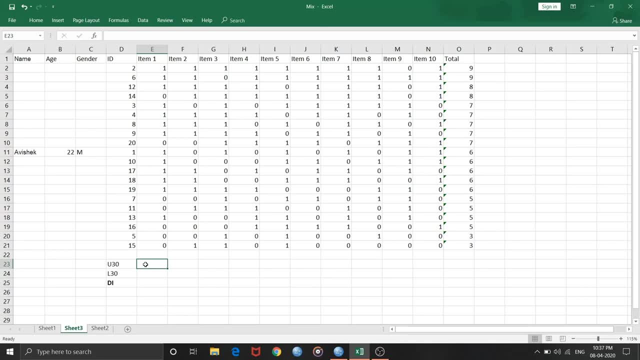 in first 30 cases, sorry, first 30 percent of cases, that is, first six respondents. how many are getting the this particular item, that is, item one, as correct. so for that all i have to do is i'll put equal to. i'll have to use formula: some information. i'll double click on that and then 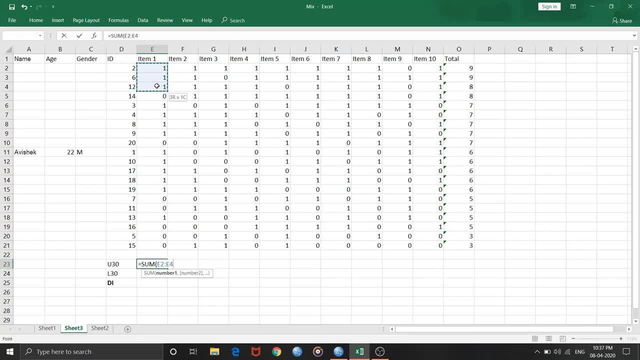 i'll have to select first six response responses. but, uh, respond response is given by six first top scorers, so i can select over here three, four, five and six. okay, so these are six respondents. now i'll complete this bracket. i need one more bracket above it, so because since it is going to be one like complete formula, so i'll insert one. 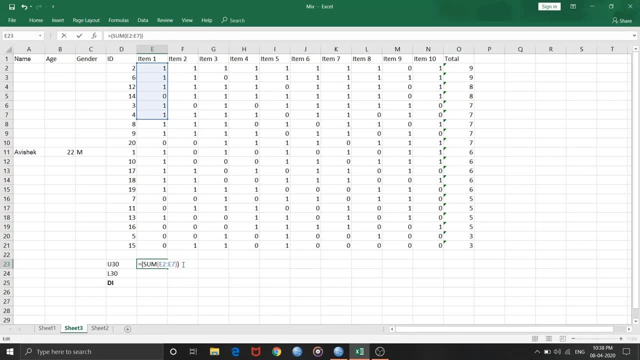 more bracket outside of it. and now i'll have to divide this value by six. i need mean of the correct responses over here. so six responses respondents are there and this is uh. there the total will be divided, or total correct responses will be divided by total number of respondents. 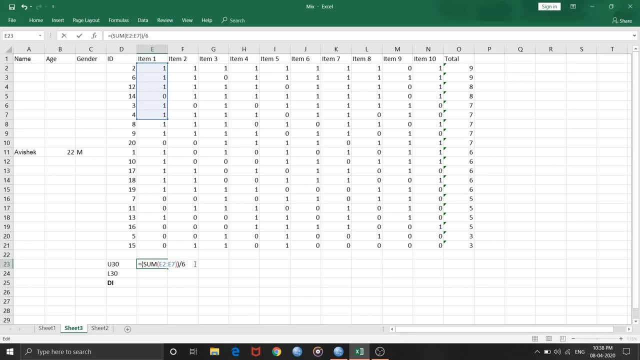 that is six. so that will give me upper 30 percent count where you can see that it is 0.83. that is, 83 percent of people scored it correct. remaining scored it wrong. now in lower 30 percent i need to check how many respondents, or how many percent of this, what percent of respondent, have solved it. 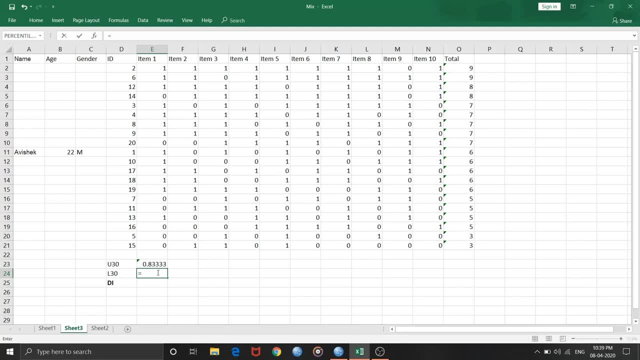 correctly, uh, incorrect manner. so i'll go again for equal to some double click on that and now i'll have to select last six respondents. so carefully, i have to select last six, so these are my last six responses. if you see, i'll complete this bracket. put one more bracket outside of this box. 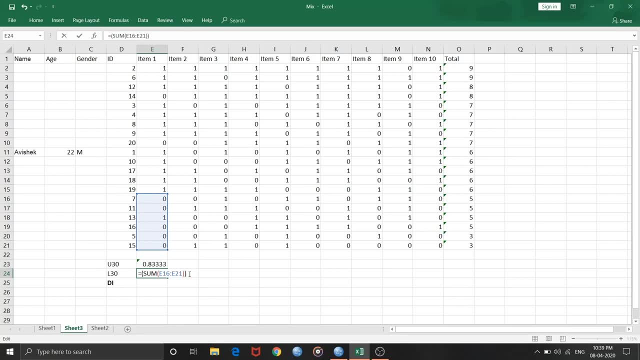 outside of this formula. and then i'll have to divide this also by six. that is total number of respondents. that is six in my last 30 percent respondents. so this will give me L 30. that is lower lowest 30. we can say low, lower group and upper group, and now discrimination index is nothing but. 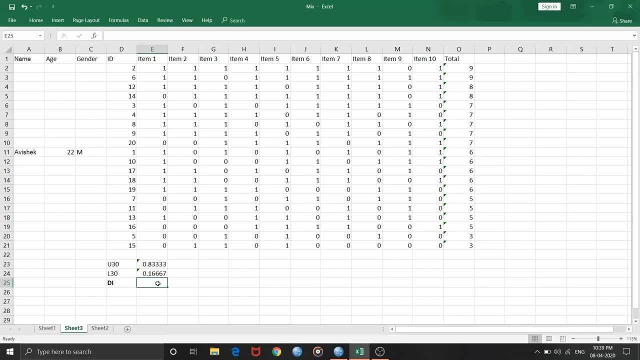 difference between u 30, that is, upper group, and lower group. so I'll simply put formula as equal to this value, that is u 30 minus lower group, that is you thought L 30. I'll click on Enter and see this is discrimination index. sorry, discrimination value for this particular first item. now, if I select, 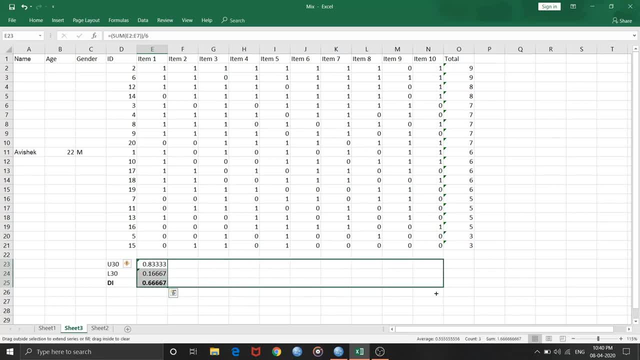 all these three and write these for all the items. I'll get item discrimination index for all the respawn, all the items over here and now. if I want discrimination index in percentage, now it can, ideally it should range from it. it it ranges from minus one to plus one. but in some like uh, in some uh- you know books- you can see that discrimination index. 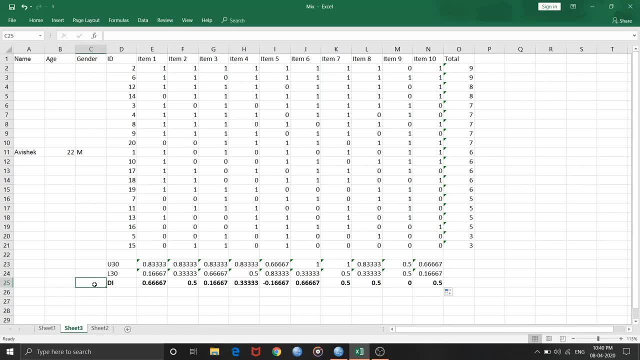 is actually given in percentage, so you can for, for. for your ease, you can actually multiply these values of the discrimination index by 100 in order to get percentage that you can, even here you can do that. i'll call it as di percent and that will be nothing, but this value will be multiplied. 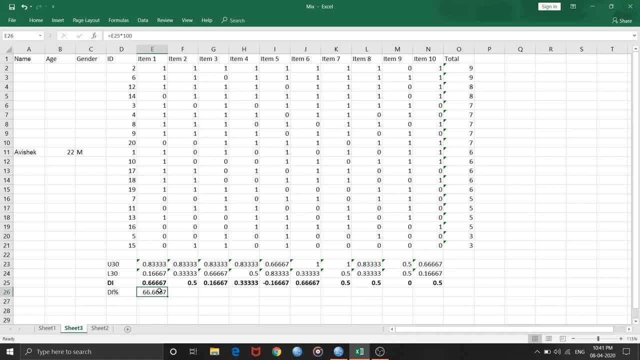 by 100 and now it is in percentage and if i drag this i'll get percentage for all the respond, all the items. so you can have it in percentage or you can have it in decimals. so in decimals it will range from minus one to plus one. in case of percentage, it will range from minus hundred. 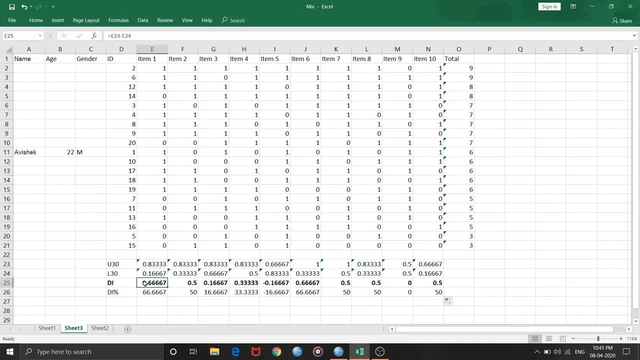 to plus hundred percent. okay, so now this is how much this item is discriminating between the respondents. now, um, rule of thumb, over here is point zero to uh 0.2 are actually not discriminating much, so those items can be actually removed from your data. 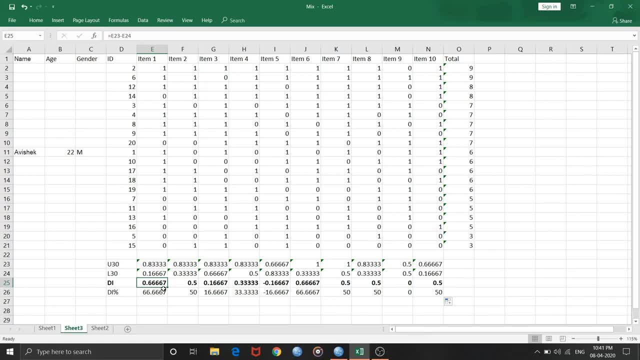 from a scale, whereas items having discrimination index of 0.2 to 0.4 are starting to become discriminating, whereas items which has value of item discrimination uh more than 0.4 are strongly discriminating between the respondents. so in this case you can see that uh, as per. 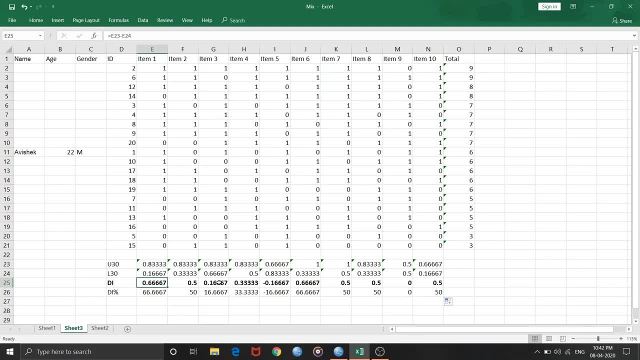 this cut off strategy. if you go for like point above point two, i will select items till one. so below point two, i can point out that this item three is having a low value. on the other end, item five, we also producing some sort of negative value over here and one more item nine is also producing 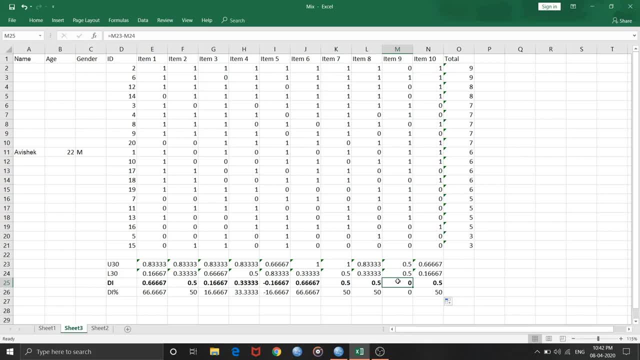 very low value of zero. so these three items are actually not- uh, you know are are not discriminating much between the highest and lowest uh scorers of this point of the data. so you can actually remove these items. so item three, item five and item nine are actually, uh, not producing. 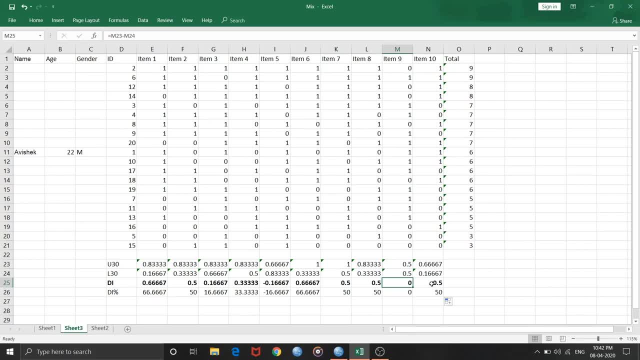 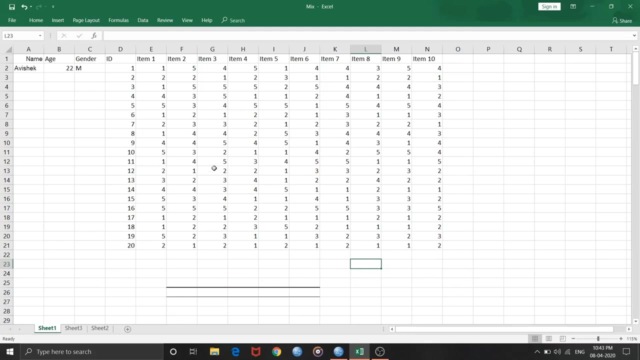 satisfactory. uh, you know discrimination between respondents. okay, so this is easy in case of dichotomous item. what if you have like at scale? so in this second part we will see now how to perform discrimination um item discrimination in case of likert scale. now, in likert scale there are no as such right or wrong responses. now this: 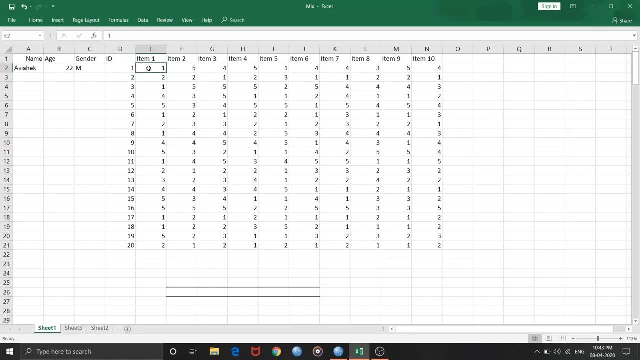 is another fictitious data i have wherein i have likert scale i have used. so the least possible score on an item is one and maximum possible score on each item is five. so it is basically a five point likert scale ranging from one to five as the responses. so there are no right or wrong responses as such, but 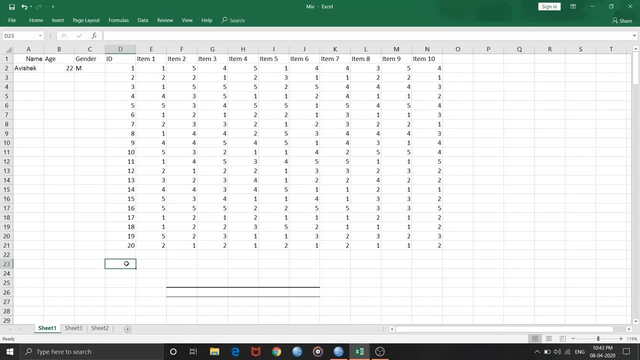 now this: this is um a likert data, and again i'll have to follow same sort of similar steps over here. i'll have to write total. we will be using kelly's suggestion only, that is 27, top 27 and bottom 27 of cases. for that i need total scores. so for total i can simply use this summation formula. 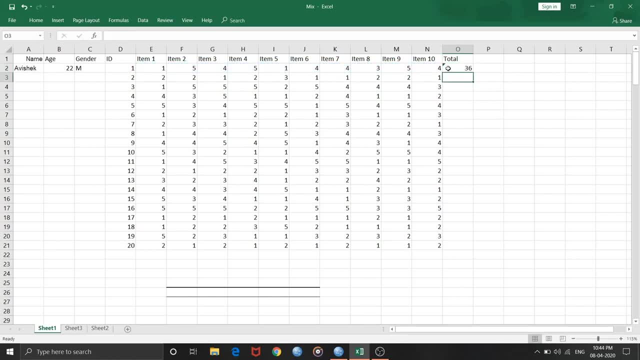 and i'll select all these items till 10th. this gives me value for the first respondent drag down for all the respondents. so this is total value i have. now i need to sort this data in descending order, that is, from highest score to lowest score. in order to do that, i'll 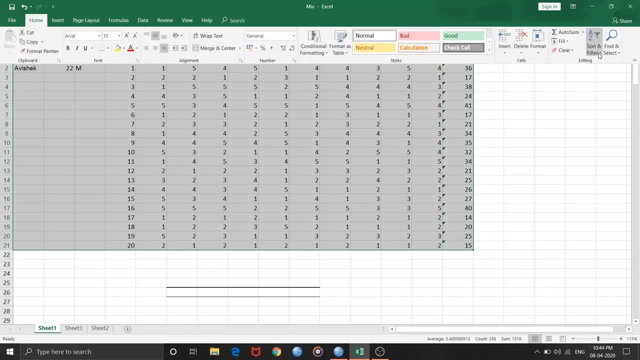 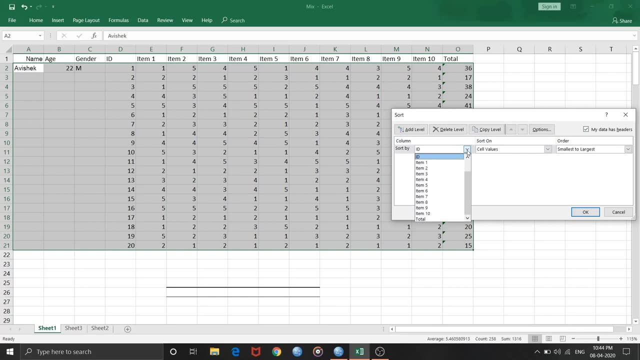 have to select entire data, go in home, sort and filter and custom sort my data. now again, this box i have already checked, so i'll have to sort my data with help of total scores and i need to have it from largest to smallest. so i'll click on that this. 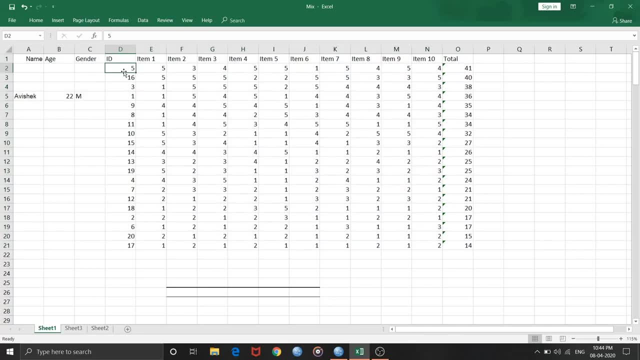 will sort my data and now you can see that fifth respondent, id id50, is actually scoring the highest and id 17 is scoring the lowest value, which is uh 41 and 14 respectively. now, in this particular data again, see, basically we are going to use similar sort of formula, but 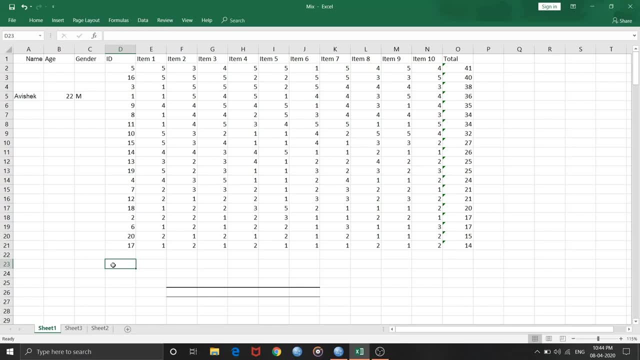 then a slight difference is there in the last step of it. so we will again go for for you now in this, in this case particularly, we will be computing mean for the upper group, mean for the lower group, and then we will be subtracting upper mean from lower- sorry, lower mean from upper mean, and we'll 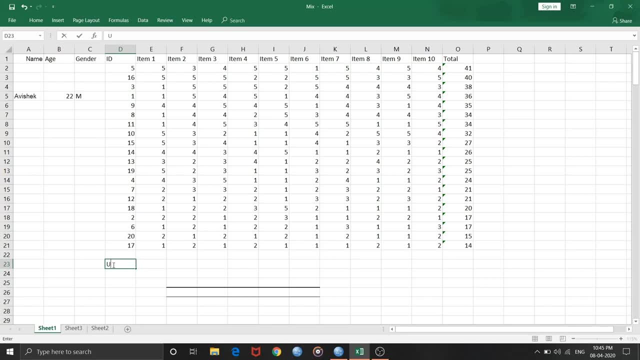 be dividing that subtraction or result by maximum possible score on one item. so we will step by step do that in this. first we will call it as u mean, that is upper mean, upper group mean, then l mean will be lower group mean, and then i'll be interested in discrimination index, which 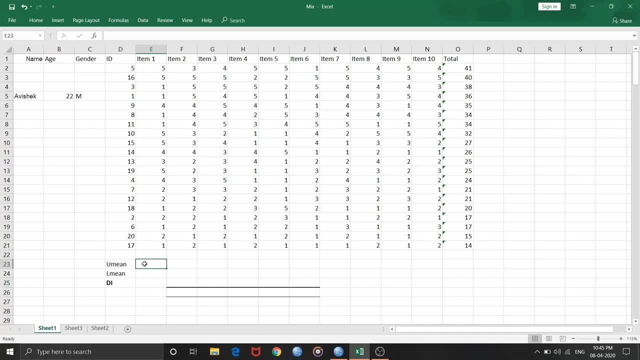 shall range from minus one to plus one, in the same manner that it has ranged for the dichotomous items. now, in this particular- um you know, data- again fictitious data- i have 20 respondents only, so i can either stick to five or six, as described earlier. that consists of 30 percent, so i'll stick. 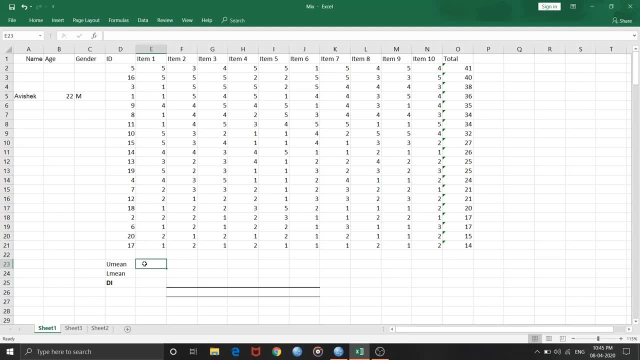 to six respondents. so in in this particular case, six respondents will be there. so i need to calculate mean of the top scorers. so mean will be calculated with help of sum and we'll divide that by total number of people. that will give me mean. so basically, i'll put equal to, i'll put sum. 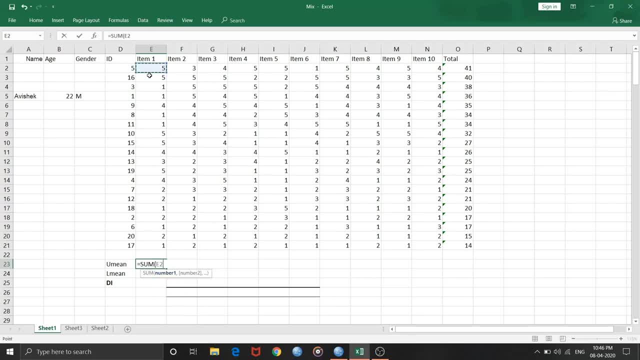 so i'll summation of first six responses. so three, four, five, six. okay, so you can see that i have selected first six responses. i'll complete this bracket, put one more bracket outside of this formula and then divide this value by six, since total number of responses i have six over here, so six people are responding to. 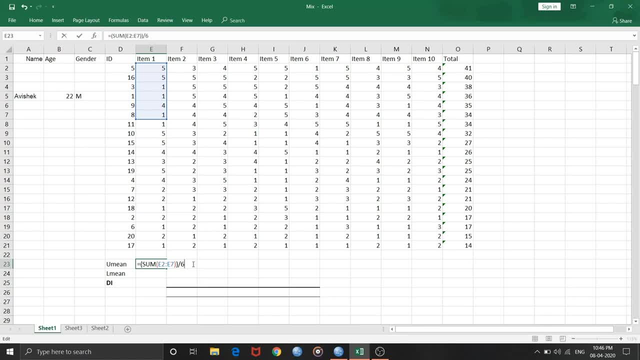 one particular, like first item in my data for my scale. okay, so this is mean of first upper scorers. now mean of low scorers or lower group. i need for that same formula sum. okay, if we select last six values, complete this bracket. put one more bracket outside of it. divide this value by six, because six 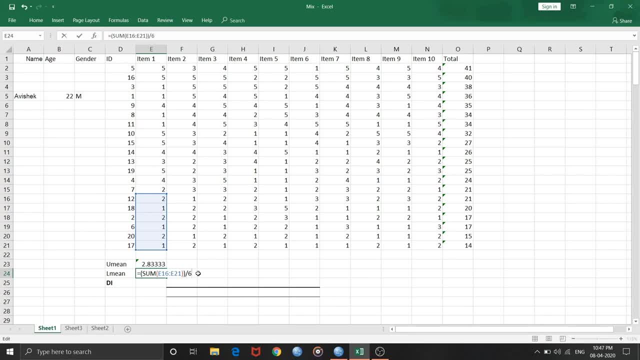 response respondents are there for the lower group. this is giving me lower group mean. now, in this last step now since, like we have followed almost similar steps so far, but in di discrimination index we simply need not to subtract values, but we'll have to divide by maximum possible score, two. in this particular case, that will be. 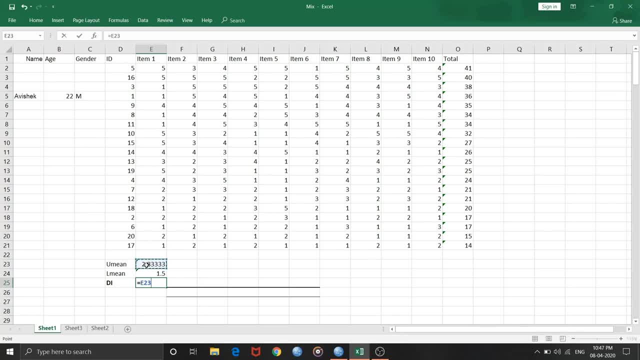 equal to this value. that is, upper mean subtracted like. lower mean will be subtracted from upper mean. basically put brackets and divide this value by five. now, this five is not number of cases, but five is maximum possible score on one item. it's essential to divide it by now. this gives me 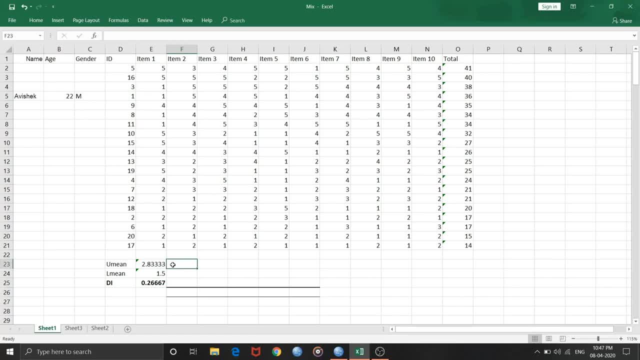 discrimination value for this particular item. now i need to simply drag this, these three values for all the remaining items. it will give me discrimination index. now see again. here you can see discrimination index, whereas in this particular example now item item five is pretty much on the borderline, that is, for my cutoff criteria is 0.2 and above, so it's still meeting. 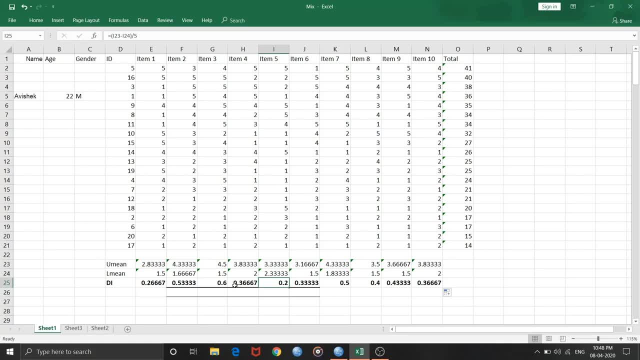 the criteria. in other cases it's pretty okay. so, yeah, still, like, item five is uh, you can, you can remove item five if you want to. apart from item five, other items are actually pretty much, uh, you know, doing well in discriminating between the high scorers and low scores. now, um, since this, um, this is essential to know that it's not just 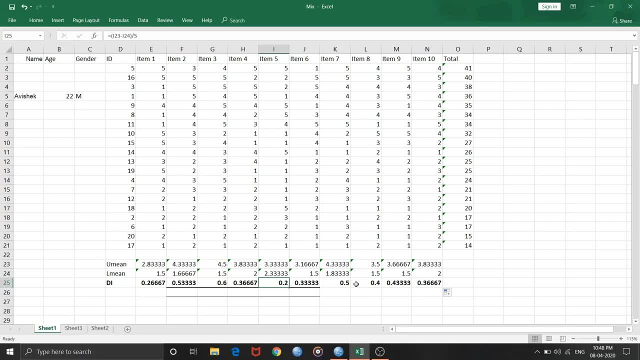 discrimination index. you decide whether to keep item or to discard it from your test. but it's not just discrimination index: you decide whether to keep item or to discard it from your test. but important is to see theoretical importance of that item. so i'll suggest you to go for content analysis. 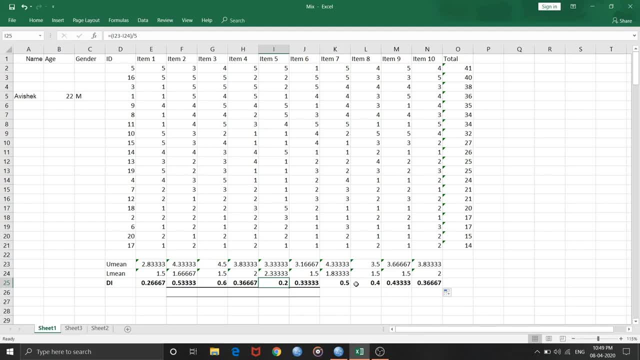 or else at least check theoretical importance of that item before deleting. if it is theoretically important, though it might not be producing a very high discrimination value, you can still- you know- reword that item and use it. so it's not just about discrimination index, but also theoretical importance of that item. 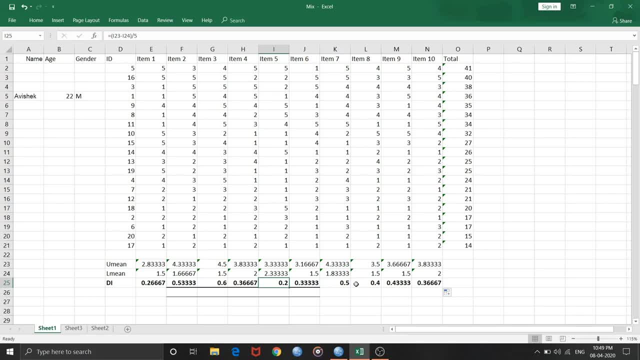 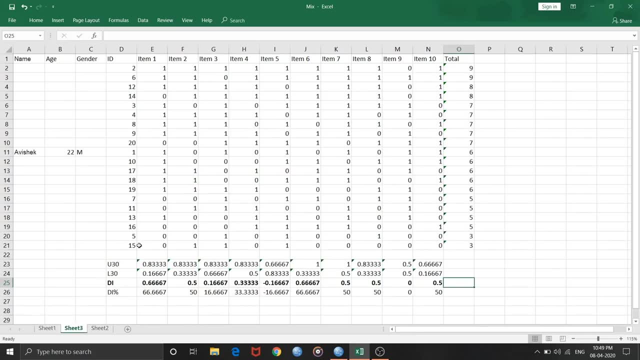 all right. so this is for uh, the like data. a very slight difference is there in the formula if you see for like a data and for uh for this dichotomous data. now, third very popular method is uh corrected item: total correlation. in this particular method, what we we, what we do, is uh. basically, it's very 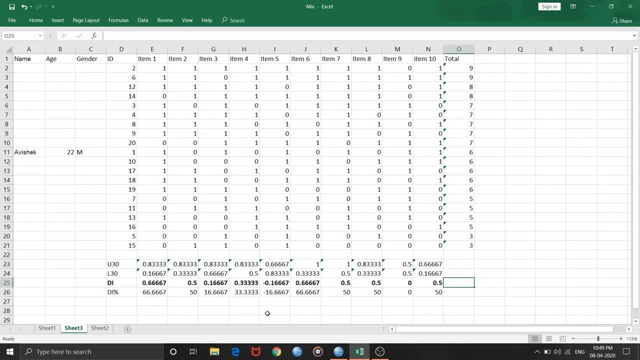 going very close again to the internal consistency reliability. so in the state of internal consistency, we'll be actually purifying our test in that. also, where we can with help of uh- certain formula will come to that- we actually purify our test. so with help of corrected 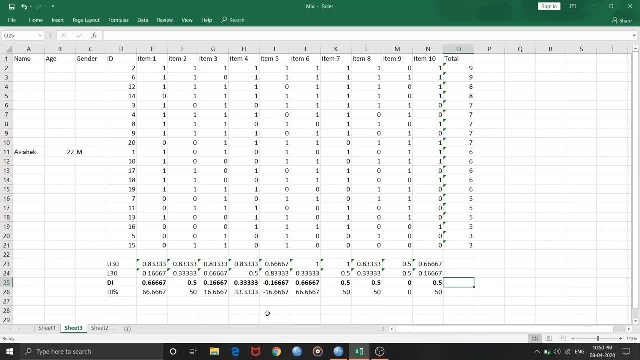 item total correlation value. we can remove certain items which are not actually homogeneous in our test and which are not actually measuring what we intend to those items to measure. so those can be removed from the, from the scale, in order to produce a good scale. so for that particular method that is corrected. item total correlation we need a spaces, so in a 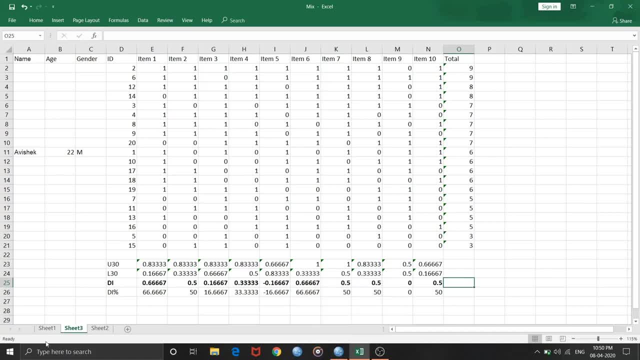 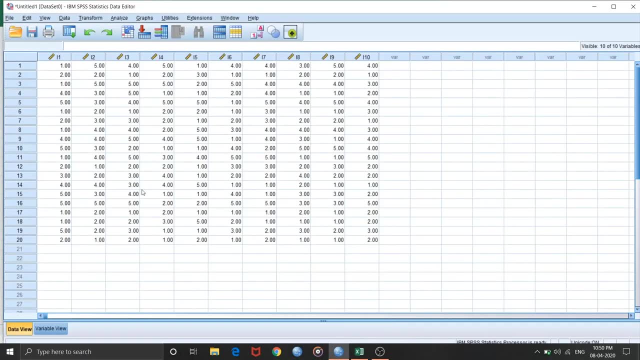 spaces. i'll simply put this: uh, like a data now in for this, like a data, we can compute it in our spaces. i'll simply copy paste this data. i have copy pasted over here already, so in variable view you can check that how i have defined these variables. 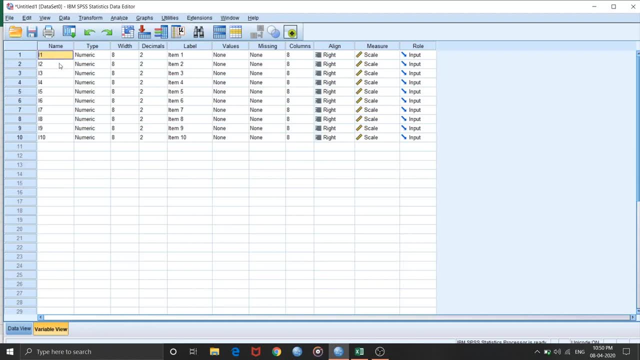 in name you can't have two different uh words, so i have coined those as like. i1 stands for item one in label. however, you can check that as well. use your creativity and you can have even space between two values. so item 1 I can completely write over here in label, but in a in name I can't do that. 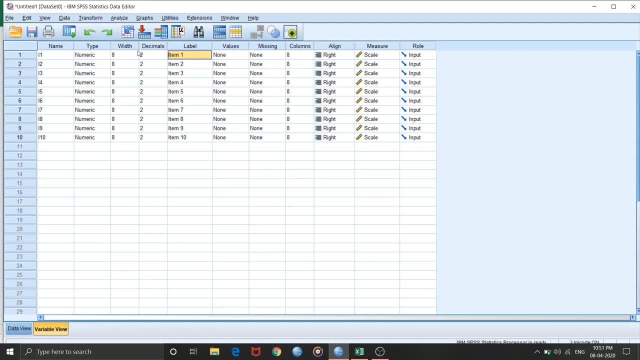 so, and apart from that, these other other values are by default selected by spaces and these values are selected by like, manually scale. so you need, when you have like a data- many authors are of this view that- or many researchers are of this view that if you have like it data, it is. it should be considered a scale. 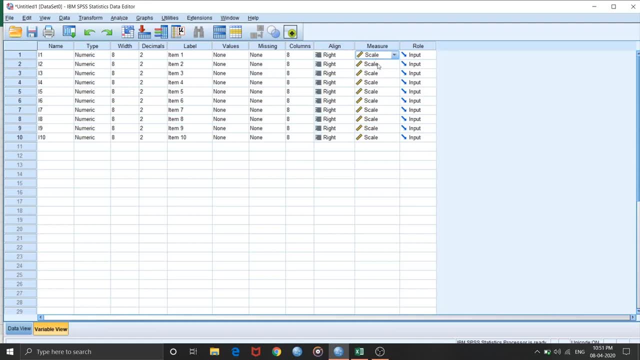 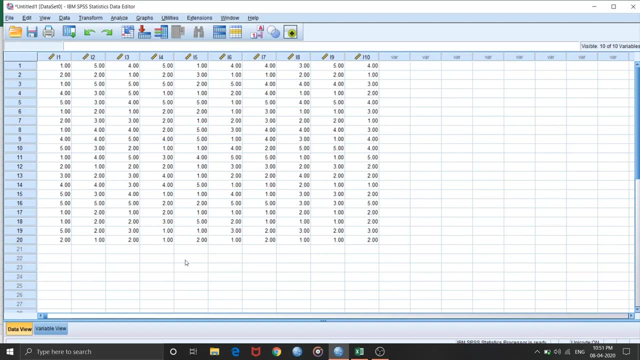 major. however, there are some differences and some people even go for ordinal data, so we will stick to scale, alright. so in data view you can see that I have ten respondent, certain items and twenty respondents in my sample. this is again a fictitious data, simply to have copy-paste it over here. so in analyze you can go. 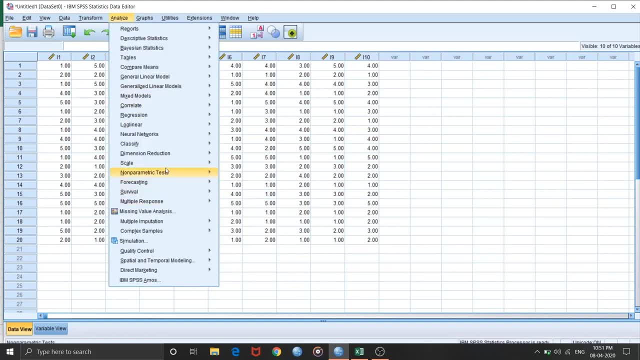 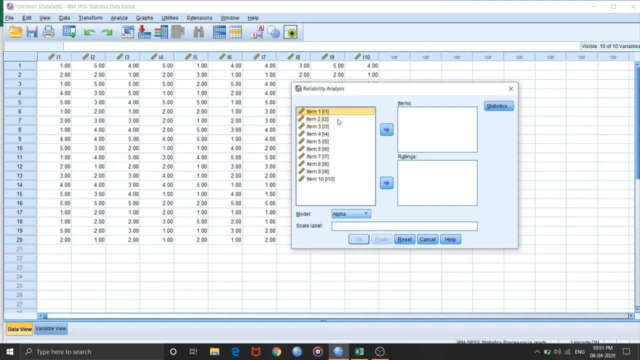 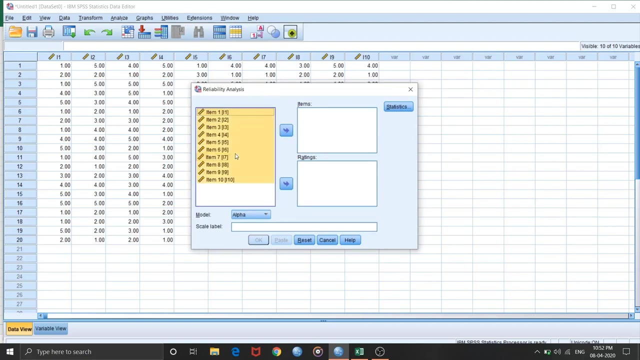 in order to compute this corrected item. Don't go away. go in scale. reliability analysis. now in this type of dialog box will appear over here. there are total 10 items, so I can select all those in one go with help of ctrl A, and click on this small icon will shift my items in the second box called 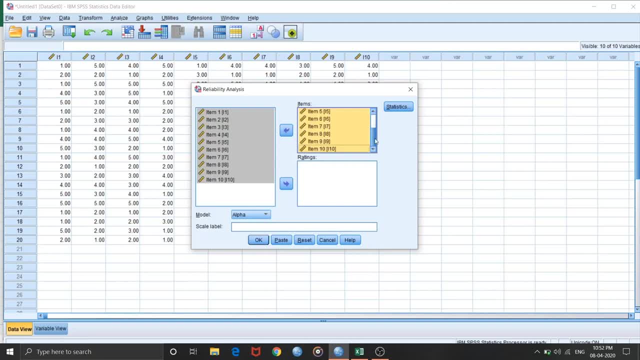 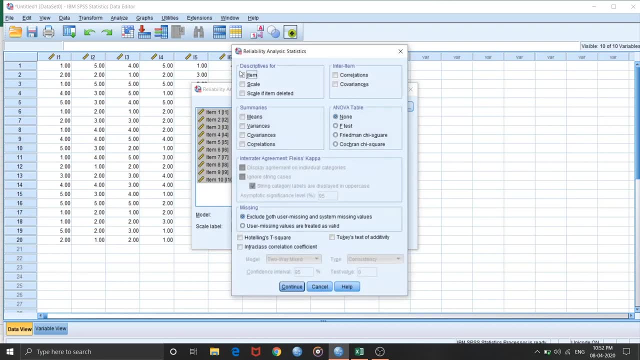 as items named as items. okay, so I can see that all my terms are. you know, I have transferred those in items in statistics. I need to check certain values in descriptives, for I am interested in all three. so item scale and scale if item did this last function, scale if item deleted is pretty. 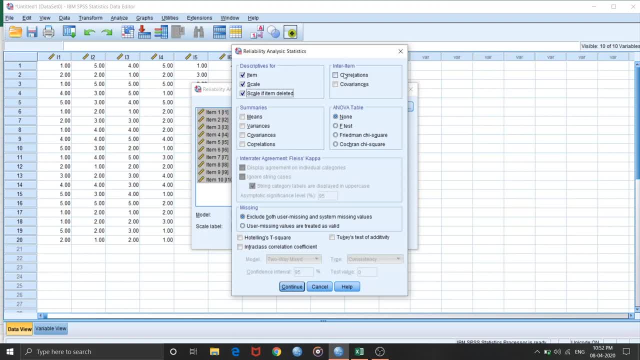 interesting. we'll see that. and then I am interested in inter-item correlations, so I'll click on that. apart from these three values, I'm not interested in any other value, so I click on ok. in model, I'll suggest you to go for alpha only, since it gives you internal consistency, apart from 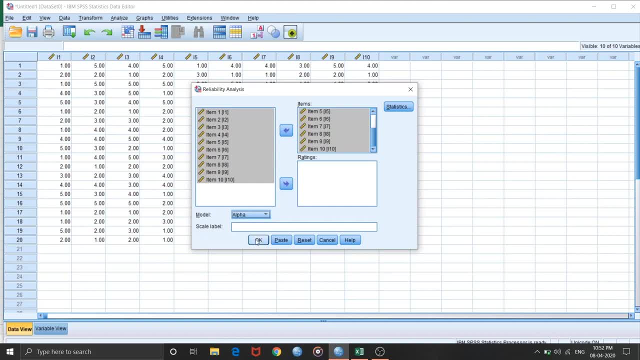 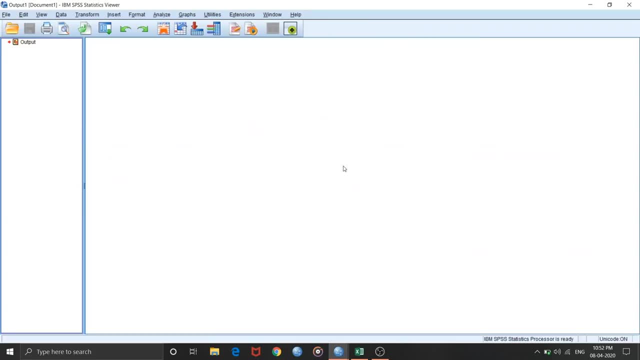 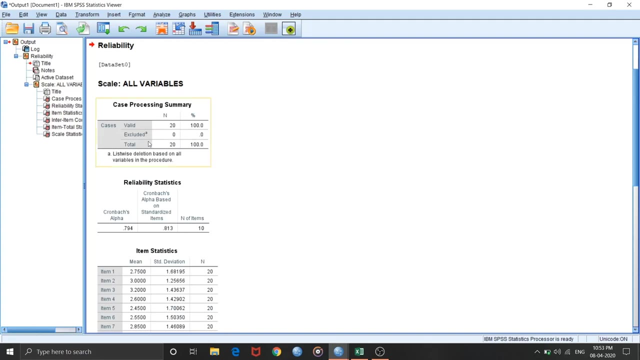 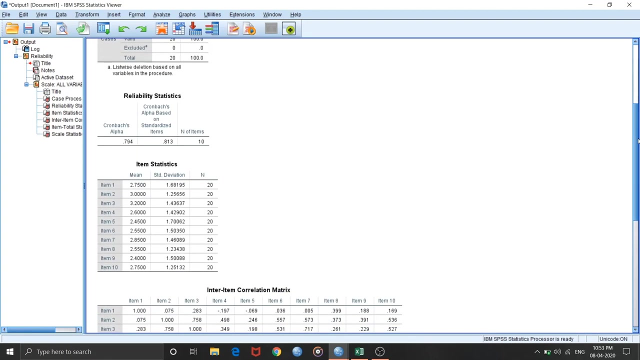 the, the total item- total correlation and corrected item: total correlations. so click on ok. this will generate your result. so in output you can see that um these values over here. then cases: you can see that total number of cases are 20. so all cases are valid in my data here you can see that. 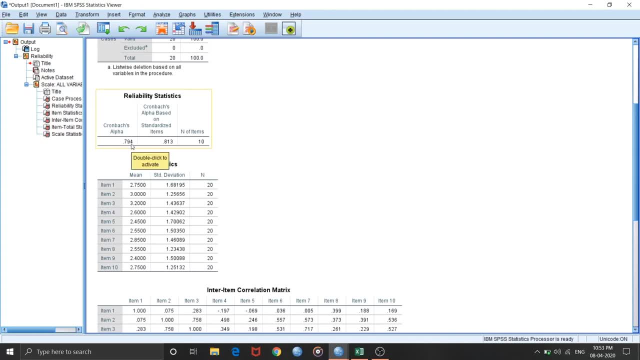 cronback alpha is 0.794. for crown back alpha, again, there are different cut-offs given by different authors and researchers, but then very popular one is that it should be above point seven. any value below point seven is questionable. above point seven is acceptable. above point eight is. 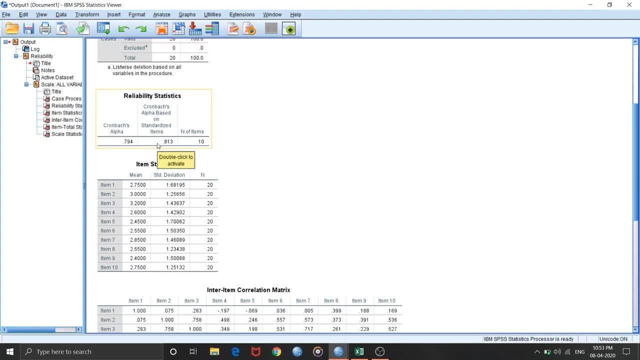 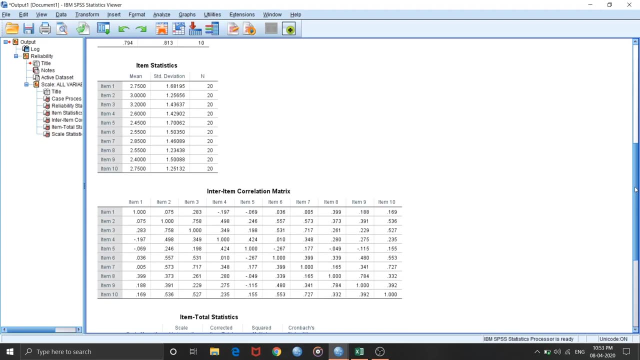 good now our values very close to point eight, but still it is not exceeding pointed. we'll see that, uh, what to do about it later. and in in item uh statistics you can check mean and standard deviations for each item and then you can see that the next item is the name of this item. 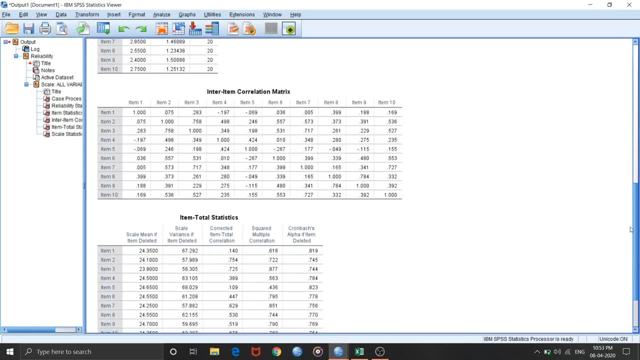 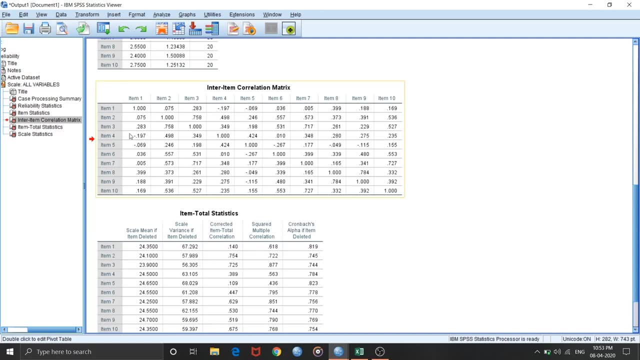 and n is 20, that is 20 respondents. inter item correlation matrix is pretty, actually the values we are interested in. so in item 4: if you see item 4 is negatively correlating with item 1, we should not be. the should not be the case, since this data. 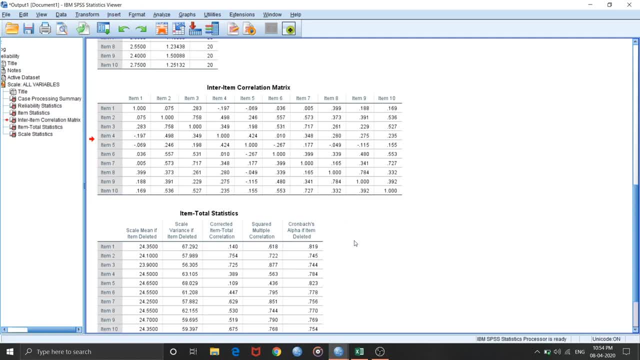 is of one theoretical construct only, so it is measuring the similar theoretical construct or the only one theoretical construct, so it should not have negative correlation between with with other items, but still it is having. so this item actually is may not be performing good, which we would be interested in to check that even item 5 is producing negative correlations. 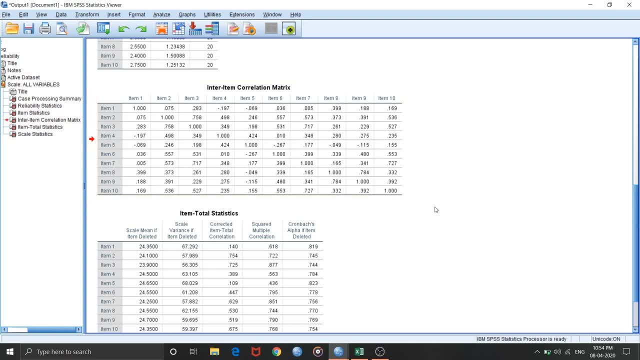 and there are a couple of other negative correlations over here. if you have item inter item correlation matrix with most of the values above 0.3, then you are pretty close to a very good correlation between item 5 and item 6, which is very good. internal consistency, reliability. however. 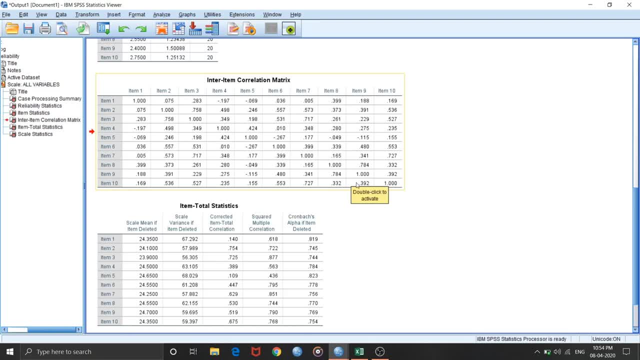 in this data you can see that there are a couple of values which are actually negative and pretty high values are, you know, there in the data, like, for instance, this particular value if you see it's minus 0.267- pretty high negative value. all right, so in this next table, 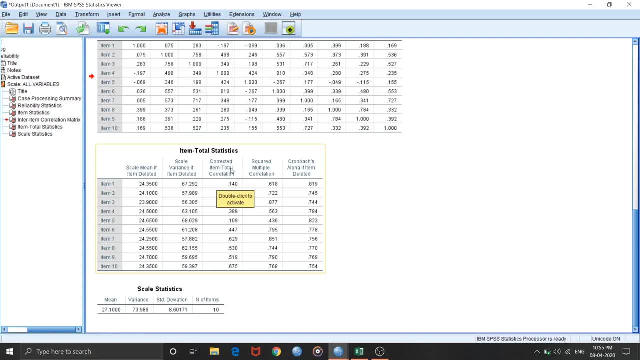 you can see item total statistics and in this third column, if you see corrected item total correlations are available for us to check. now this is the value i was talking about for item analysis. so in this case you can see there are 10 items and there are values, corrected item total correlation. first let us understand. 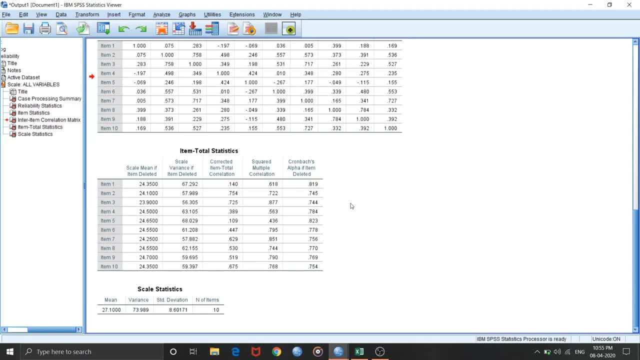 what corrected item, total correlation mean. so it's nothing but correlation of like. for instance, let's say this: first item, so first item, that is this. this value point one, four, zero is nothing but correlation between remaining nine items. total of remaining nine items, that is one, consists of one column and then 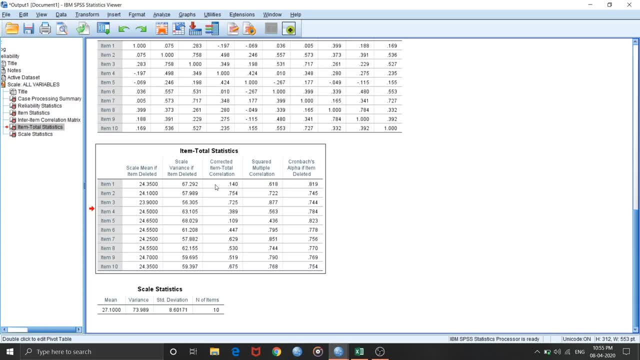 the second column for correlation will be responses on item one, so responses on a particular item and responses on other remaining items collectively. like these, two values will be correlated and correlation coefficient between these two columns will be nothing but corrected item total correlation, now corrected because this value of one item or values or scores. 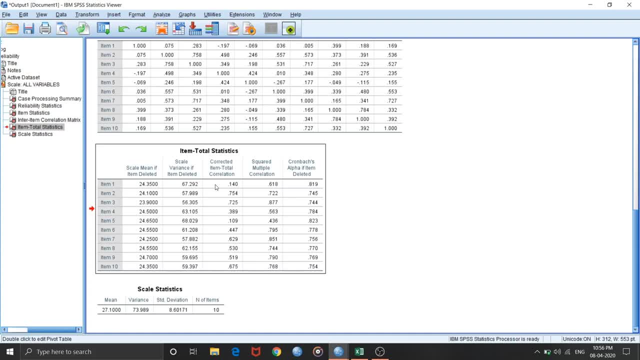 of one item are removed from the data and that are being correlated with the remaining number of items. in this case, there will be nine remaining items. so that is correlation between these two values. now, if you see, again, there are certain cut-offs over here. so, as per, like many researchers are of this view, 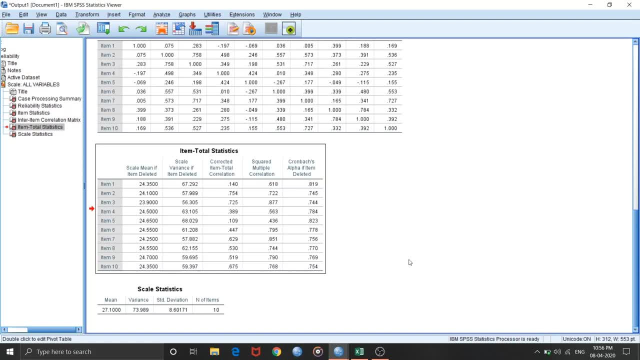 that it should range between 0.3 to 0.7 ballpark. so it should be above 0.3 and it should not be above 0.7. so in this particular case, if you see, item one is low and whereas item five is also producing very low total item item total correlation. 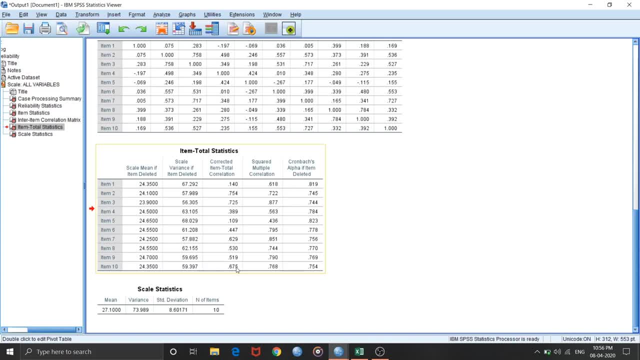 corrected item: total correlation. apart from that, other items are doing pretty well this. this particular item, two and three are actually scoring above, or having values above, 0.7. now we can actually start deleting these items, but i would suggest you to not to delete multiple values at a time, because once you delete one particular item, it is bound to change. 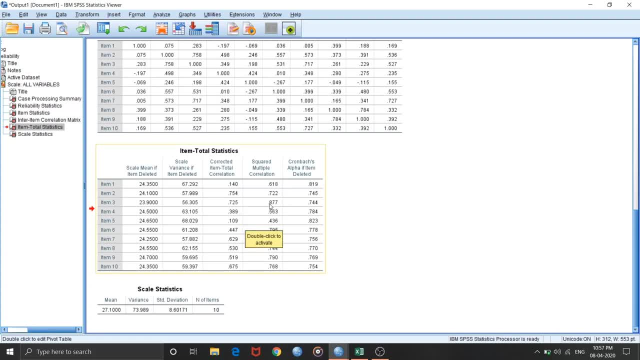 other values too, so you won't be able to see how other values are actually changing now. for instance, this value is pretty close for item third, while your 0.725 is pretty close to seven. it can even get reduced if you delete one of the items, so need not to delete directly. 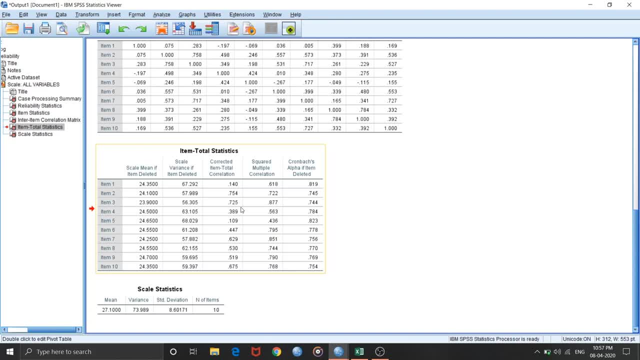 item three as well from the data. so, step by step, one or two items i would suggest to delete now in this particular case, i will be deleting one by one- and the. we can now basically delete those two. now in this particular case, i will be deleting one by one now in this particular. case, i will be deleting one by one and doing the same thing, i will suggest you to delete the two items selected, and so you need to check out. you must be clear of any additional グ constraint. so in this particular case, we have zero point seven, point 2, because don't. 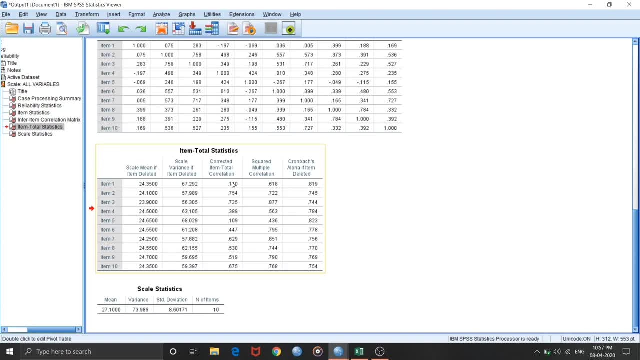 so let us start doing that. so first item I will delete as it is producing the one of the lowest values or as you can go for. actually, I can delete this fifth item. yes, it is producing the lowest value for my in my data and you can see. 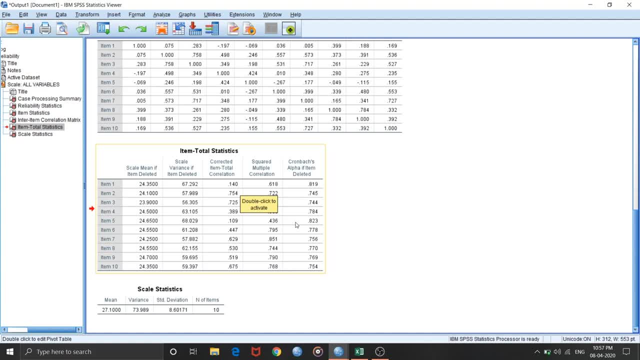 that once I delete this particular item my cron bag alpha will be improved and we shoot up to like 0.823, which is again good cron bag alpha, or that is internal consistency. that is a point above 0.8. so I'll delete first item 5. 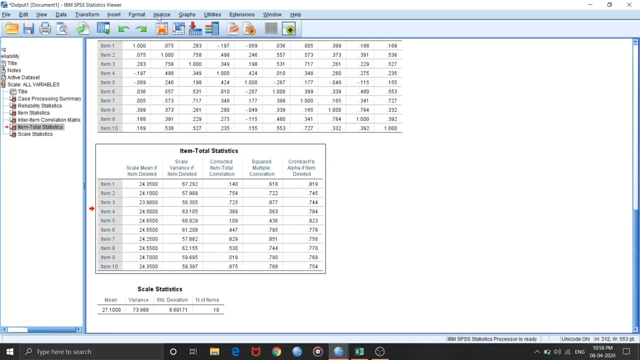 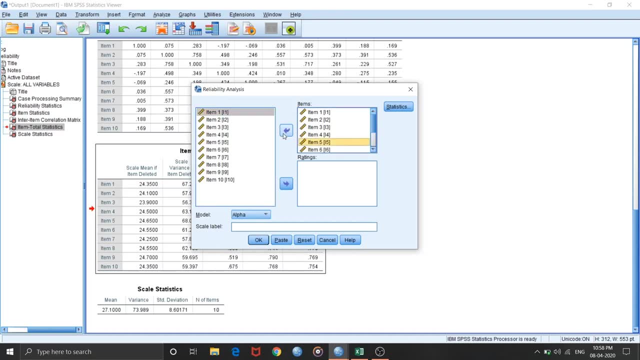 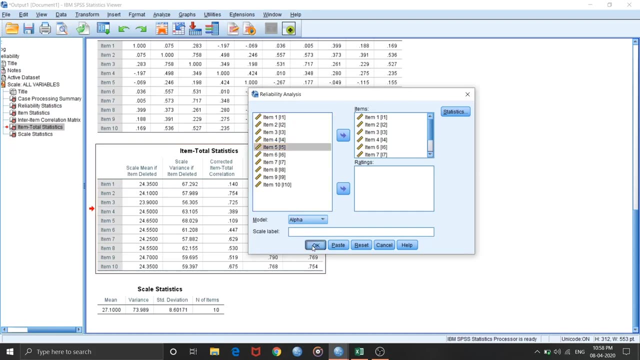 from my data and let us see other remaining values too. so go in analyze again: scale reliability analysis. I'll simply put this item out of this box. so item 5 has been removed. you can see this item 5 producing low value and click on ok. this will generate output. now you see that cron bag alpha is 0.2. 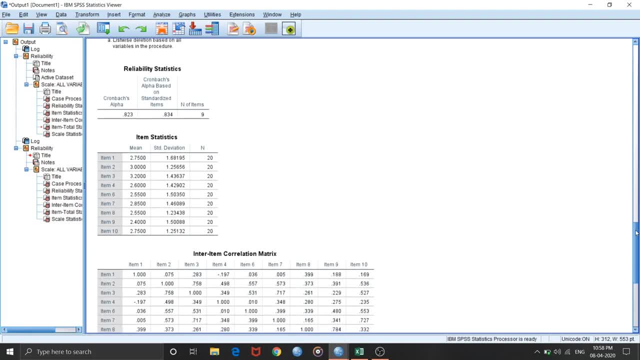 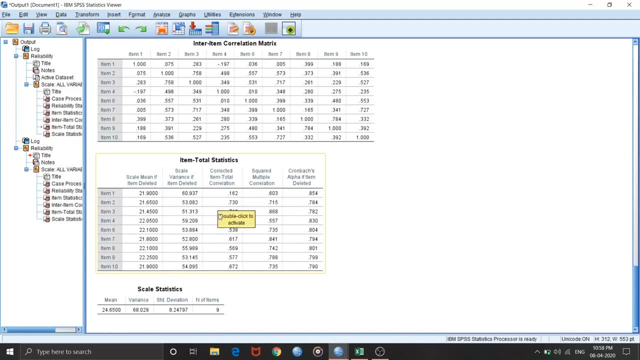 823, which is high, which is good value. now you see this, these values. now get item 3, if you see it is slightly reduced now still will not touch that item, whereas item 1 now is the case to remove since it is also producing very low. 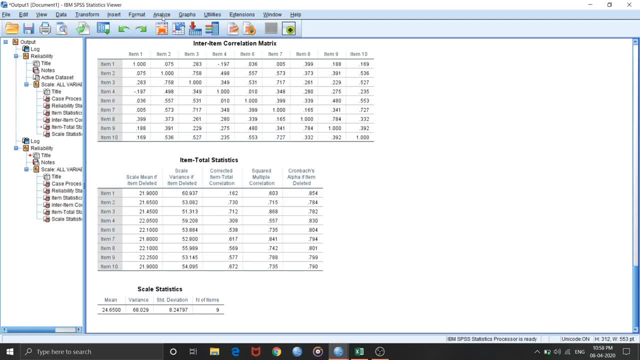 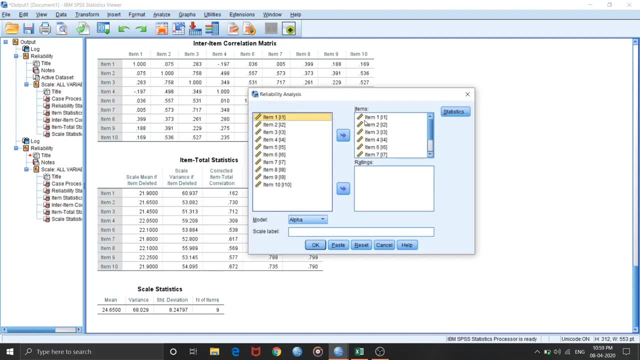 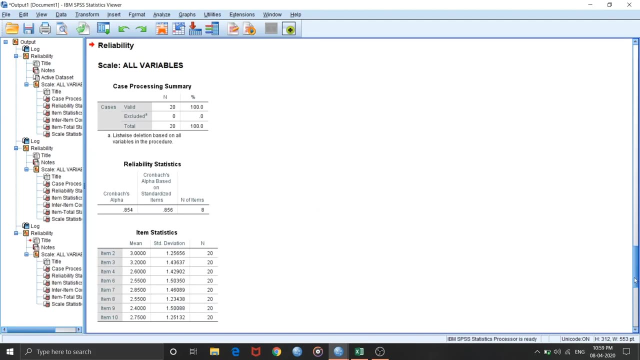 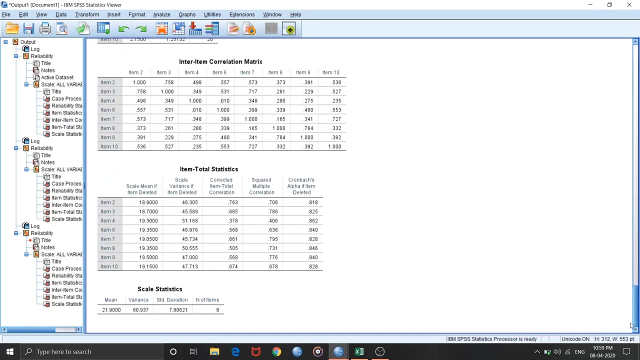 value. so again go in analyze and we will this time remove item 1 from our data scale reliability analysis. I'll remove item 1. click on ok. now if you see that cron bag alpha is pretty high- 0.854- and item total correlations, now you can see that the item 3 is now producing lower value. 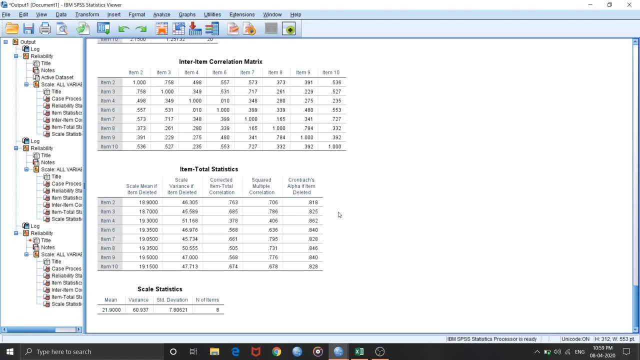 than 0.7. so this is the advantage of reducing one by one the items one by one. so now, if you see, all values are almost acceptable. only item 2 is exceeding 0.7. so in this range of point 3 to point 7, only item 2 is exceeding that. so we'll have to. 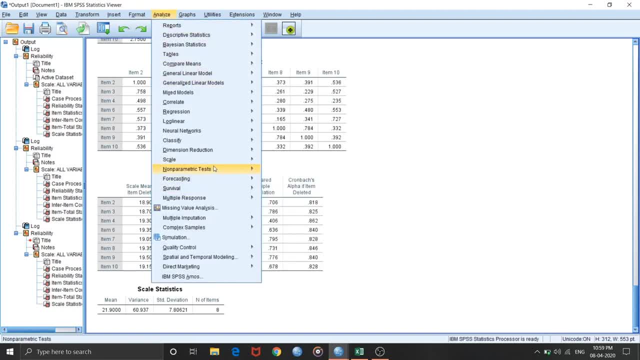 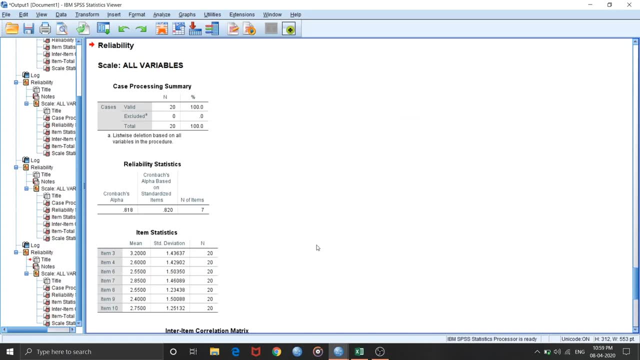 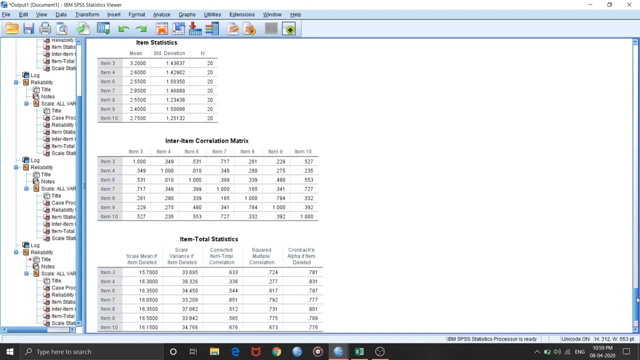 remove that item as well. go in analyze, scale, reliability analysis and item 2. this time I will be removing, and now you can see that my cron bag alpha has dropped a little. it is 0.818 now. but if you see the corrected item, total correlations, they are all now in the range of 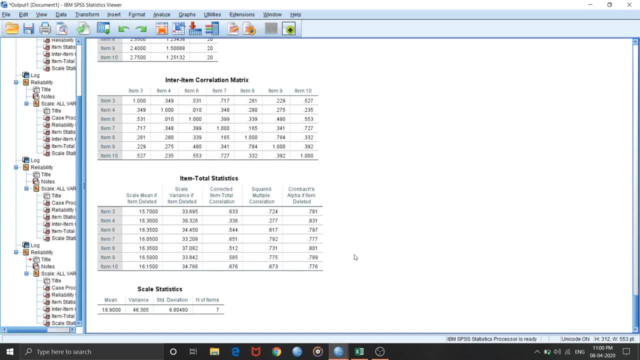 0.32- 0.7, which is acceptable range to have in a good scale and cron back alpha, if deleted, are already okay, like my values anyway above 0.8, so i'm not worried about internal consistency as such and it's producing a very good internal consistency with seven items so i have removed. 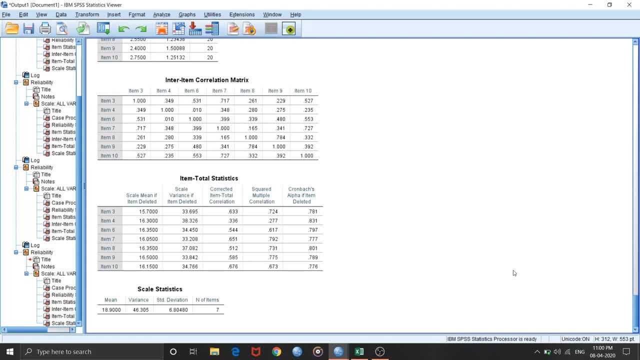 three items from my data. i'll stick to these remaining seven items now. one more caution over here is to understand that it's not just about deleting item based on the corrected item total correlation value, just like in case of item discrimination. i have seen, i've told you so. 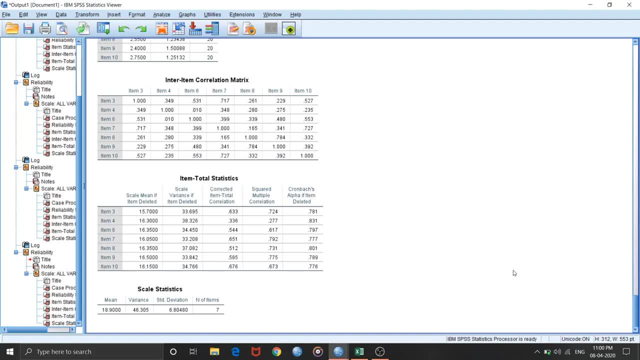 don't directly delete that item. see theoretical importance of that item and if it is theoretically important, i would rather suggest you to go for content analysis and reword that item in appropriate way and maybe after that that item can really perform good. and some other suggestions are also there, apart from continuous. now like one, one more thing. 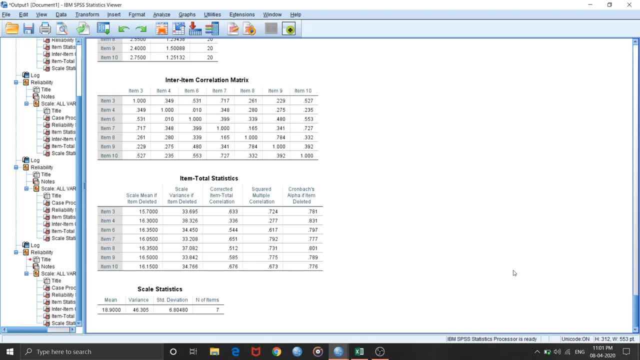 i need to explain over here is why we are deleting now many people would be interested to know that- why i am deleting values which has above the corrected item correlation above 0.7, since it is actually helping us to boost our internal consistency. but corrected item total correlation is correlation coefficient between your item of interest and the 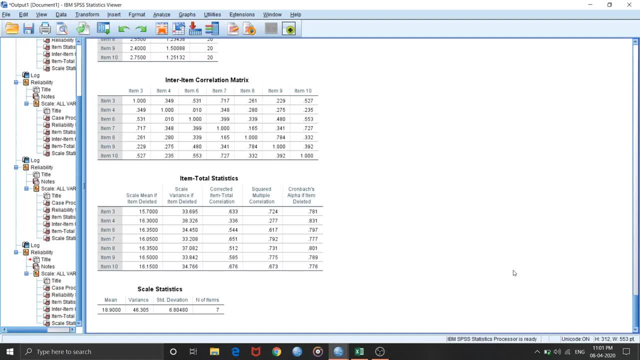 remaining items in your test. if this correlation coefficient is above 0.7, it means that more than 50 percent of variance is common between the item of interest and remaining items in your test. in other words, this item is not producing significant amount of variance and is measuring. 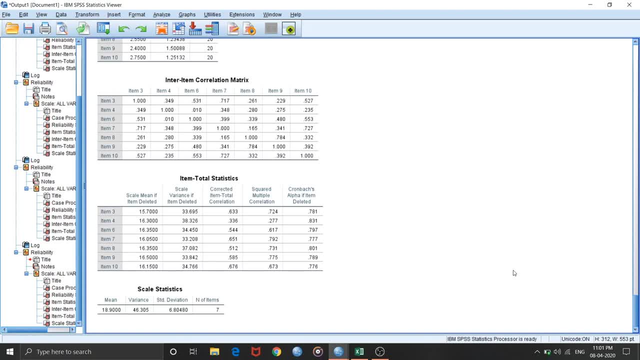 more or less the same thing what the remaining items are collectively measuring. thus corrected item total correlation above 0.7 indicates some redundance in contents or wording. in that case i would recommend you to do content analysis to decide item selection. i would encourage you to use both statistics and theory in your item or scale analysis. 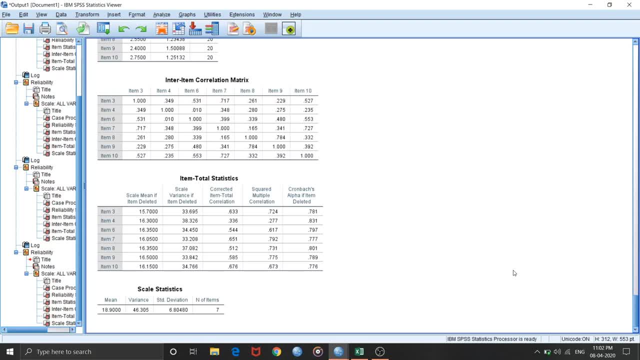 so in this video, i have shown you how to carry out item analysis with help of item discrimination method, which we have seen for both dichotomous and like a type data, and the second method i have shown is item analysis with the help of corrected item total correlation Allen. 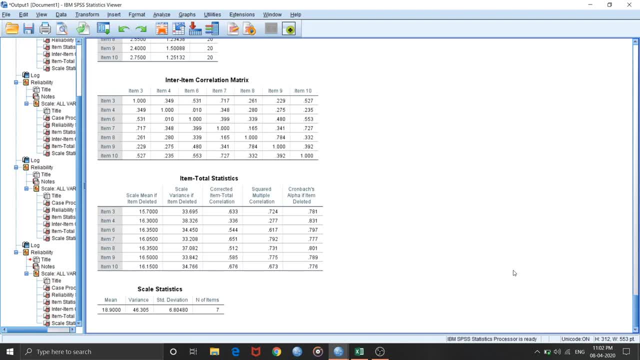 and Yen, in 1979, argued that both practices cannot be used simultaneously, that a test constructor must choose one or the other. Anastasi, on the other hand, in 1988, argued that both are important. Now I leave it up to you to perform item. 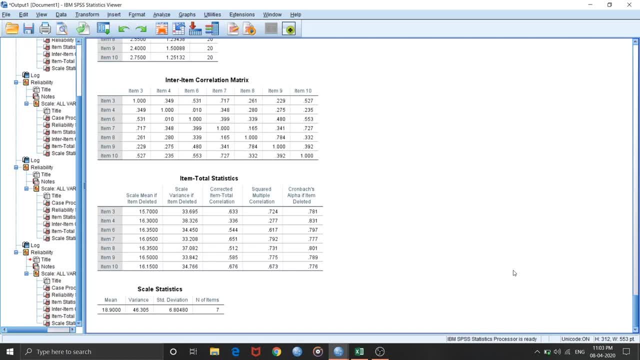 analysis with both of the methods, or to choose any one of these two If your test is generating dichotomous data and you are interested in carrying out item analysis with help of corrected item total correlation. SPSS does not provide you with KR20 as an option, So I would suggest you to do item analysis with 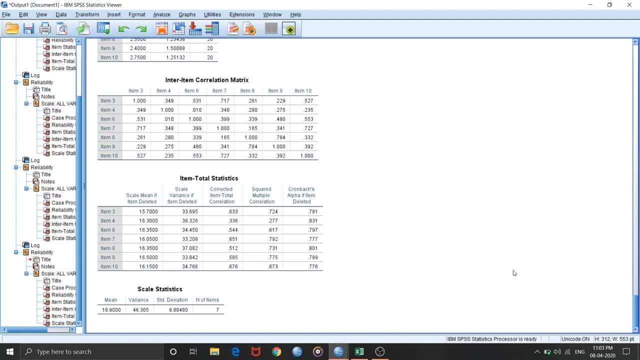 alpha only. that is scale in scale. you have to choose alpha only. So you will have to follow the same procedure which I have shown to you. So you will have to follow the same procedure which I have shown to you. So you will have to follow the same procedure which I have shown to you. 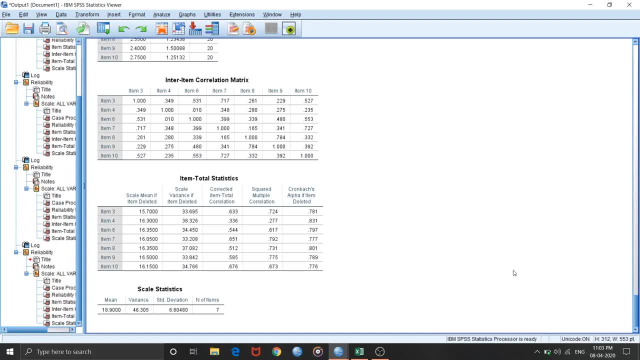 In SPSS for dichotomous data too. If you have SPSS, fine you can do that, but if you don't have SPSS, you can still perform item analysis with help of item discrimination method by using Microsoft Excel. Thank you for watching this video. 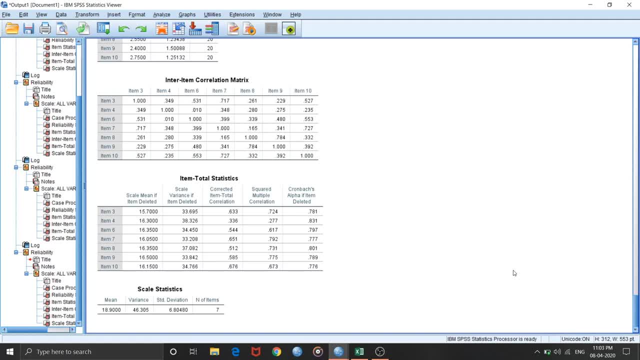 tutorial. If you face any difficulty in carrying out item analysis, feel free to contact me and I would be happy to assist you.